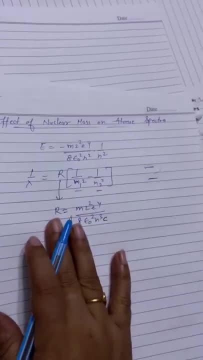 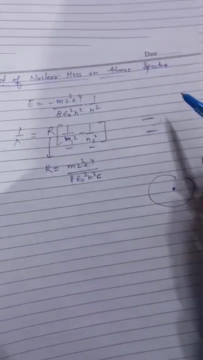 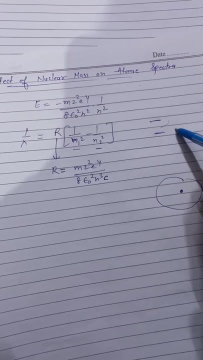 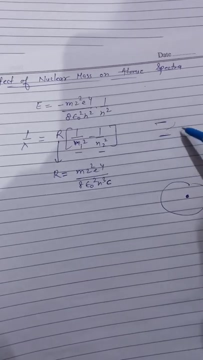 lines forming an atomic spectra. Now, if we consider the motion of nucleus as well, and like if we consider transition of an electron from higher level to lower level, then there is an emission of photon So corresponding to various transition, there are emission of photon having different frequency or wavelength, forming this atomic spectra. Now, if we consider 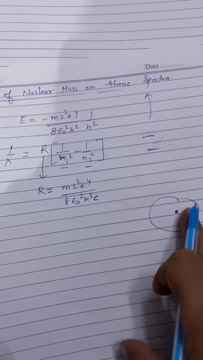 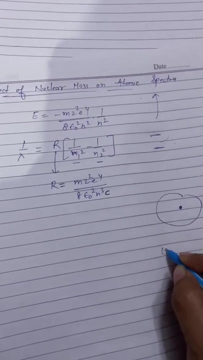 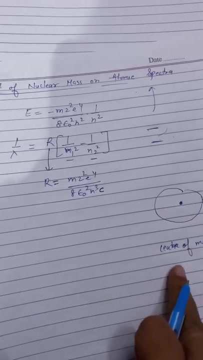 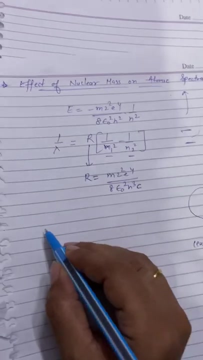 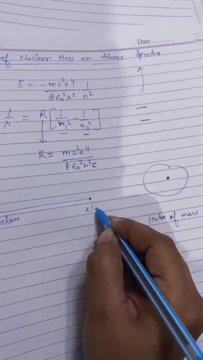 the revolution of nucleus and electron inside this atom around a common center, that is, the center of mass. that will be the center of mass around which both the nucleus and the electrons are revolving Now. so for the mathematical calculation. now we have nucleus here and electron here. Electron and nucleus are separated by some distance. 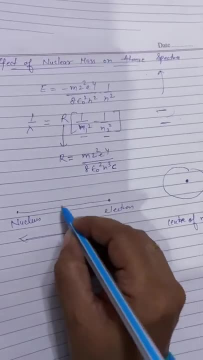 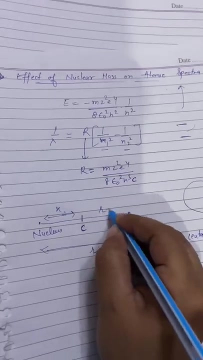 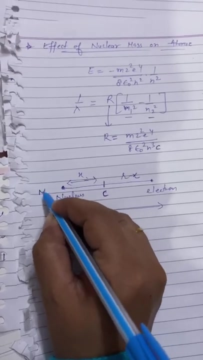 that is divided by r, and here it is the center of mass, and this distance we consider x and the remaining will be r minus x For the equilibrium condition. now mass of the nucleus is assumed as x and then mass is taken equal to r. So now we have nucleus and electron here and activity. 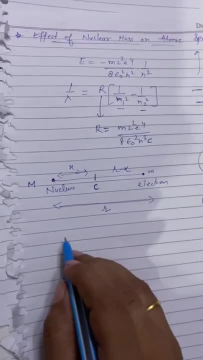 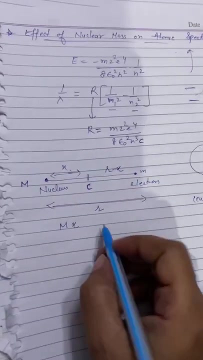 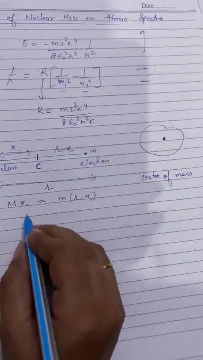 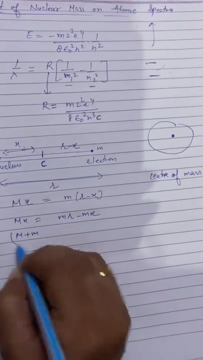 capital m and electron is small m. so for the equilibrium condition we can write m into x. that is, this distance of this nucleus from this center of mass is equal to small m r minus x. so solving this and solving this equation, m x is equal to m r minus m x. m plus m into x is equal to m r. 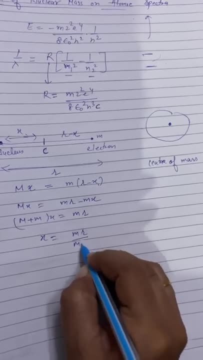 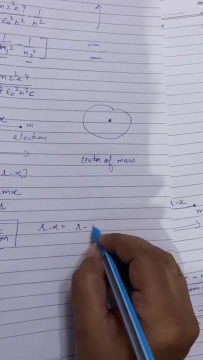 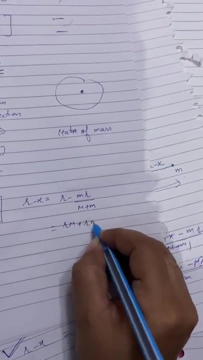 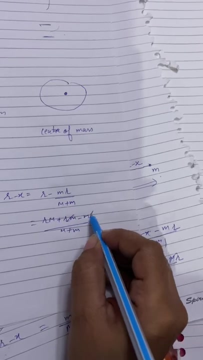 so x will be m r m plus small m. so r minus x will be equal to r minus m r divided by m plus m r m plus r m minus m r m plus m. this quantity will be cancelled out, so we will be left out with m r m. 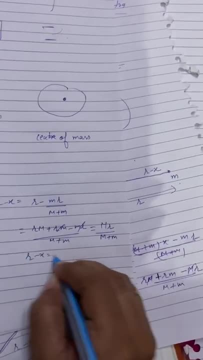 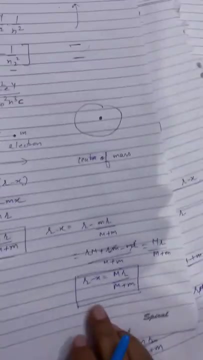 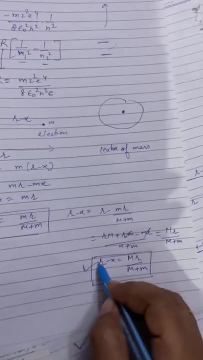 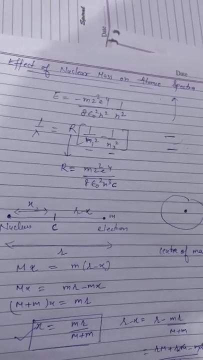 plus small m, so r minus x will be this one. so we have calculated the distance of electron and nucleus from the center of mass. this is the x and this is the r minus x. now, as both, the revolution is inside the nucleus, so the total angular momentum of the atom, as electron and nucleus, is inside the 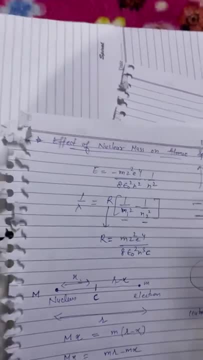 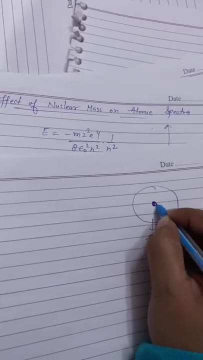 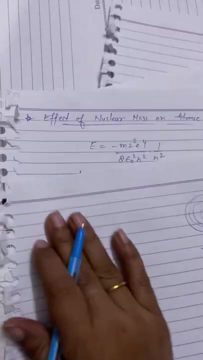 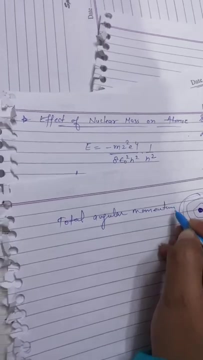 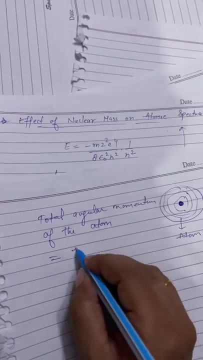 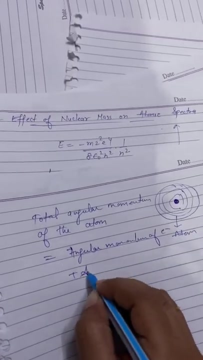 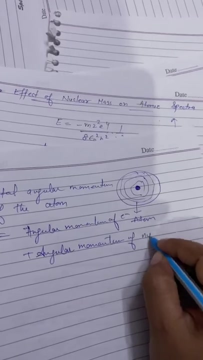 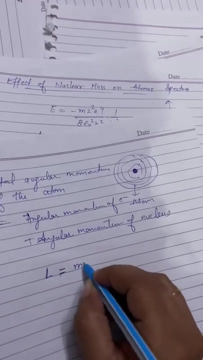 inside the atom, so the total, the atom nation. there is a nucleus around this day. now this, they are revolving electrons, so the total angular momentum of the atom will be equal to the sum of angular momentum of electron plus angular momentum of nucleus. and we know a momentum is written as: L is equal to MVR if R is. 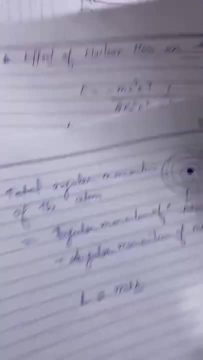 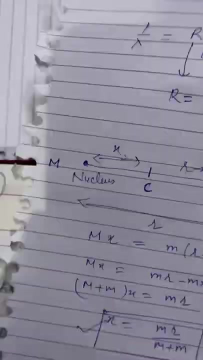 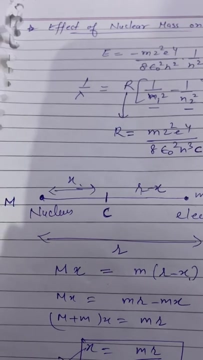 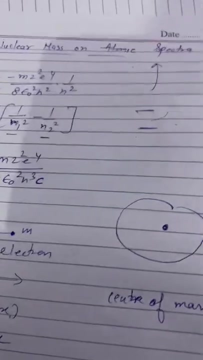 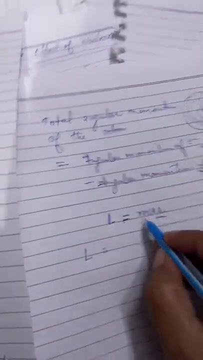 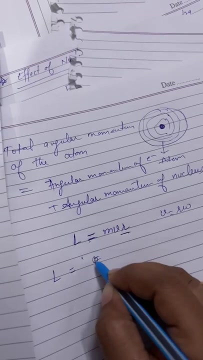 the perpendicular distance. now, in this case, in this case, if we see here, if we see here, then perpendicular distance is X. this is the perpendicular distance of nucleus from the center of mass, that is, and momentum of nucleus will be. L is equal to. sorry, we will write this equation as, as we know, V is equal to R Omega, so this form can be. 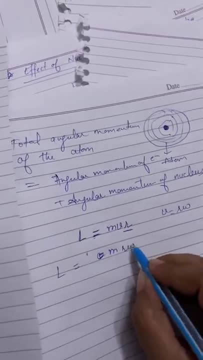 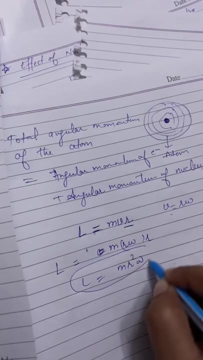 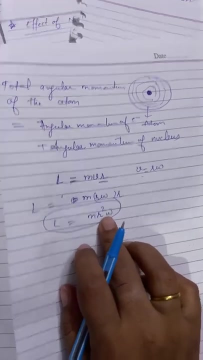 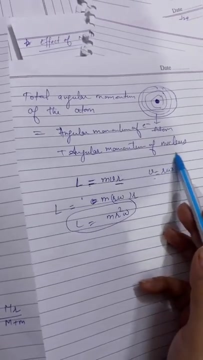 written as M V by putting the value of V R, Omega R R is equal to M R square Omega. this form is when that is perpendicular distance is R of the particle rotating particle. now, in this case, the particle here is the nucleus that is revolving a round center, center of mass. so L, perpendicular L, sorry, angular momentum.